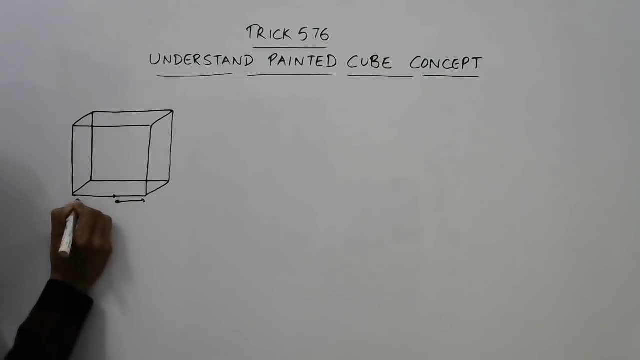 length. we have cut two equal cubes. Now this is the side of the smaller cube and this is also the side of the smaller cube. So if you have made two cubes in two lists along the length, then they will be two along the height and two along. 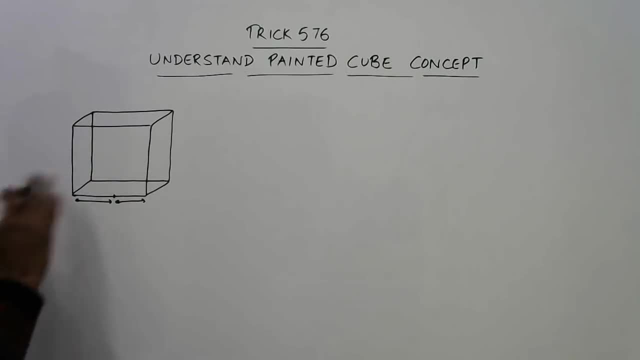 the breadth. We cannot have equal, we cannot have an equal number of cubes along the length, breadth and height. So how many sections we have made the length? The number of sections is two. So whenever we have two sections made along the length, then there will be two. qube is equal to eight cubes of 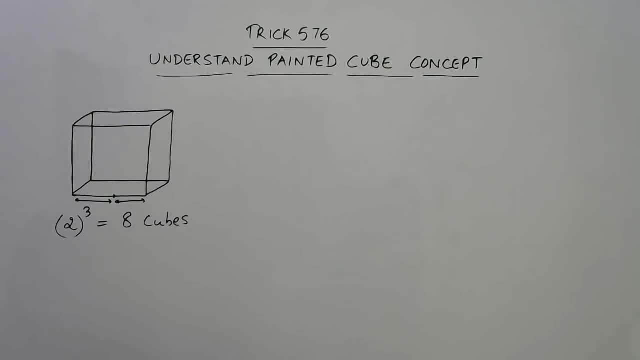 equal volume, equal length, which can be cut from this side to the other side. larger cube. Similarly, suppose you have made this section in such a way that the length is divided into three parts, like this: now see three parts. now three cubes along the length. so how many total cubes will be cut? There will be three cubes: 27. 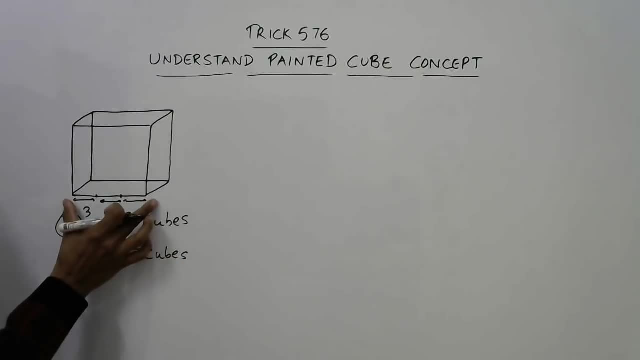 cubes. and similarly, if you divide the length into four equal parts, then four cube 64 cubes will be made, Even if the number of smaller cube exceeds 64, like, if five cubes are cut along the length, then five cube 125 cubes will be there. 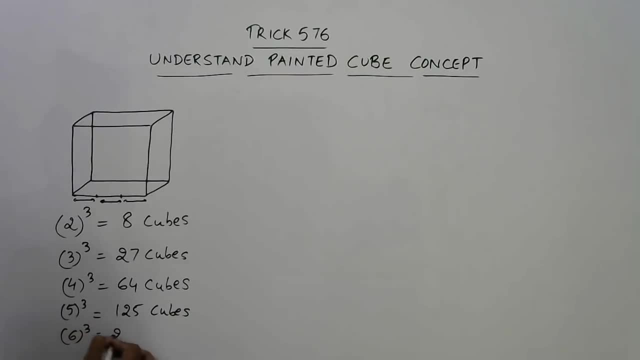 if six cubes are cut along the length, then 216 smaller cubes will be there. Now, this is the first concept. you need to know how many cubes can be cut from a large cube. It can either be 8,, 27,, 64,. 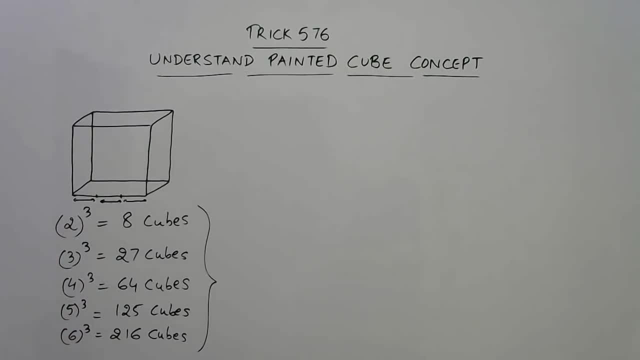 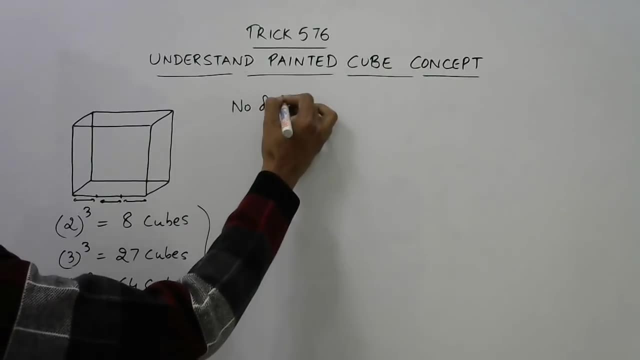 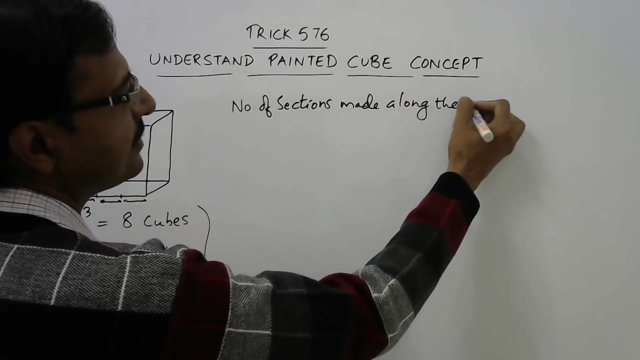 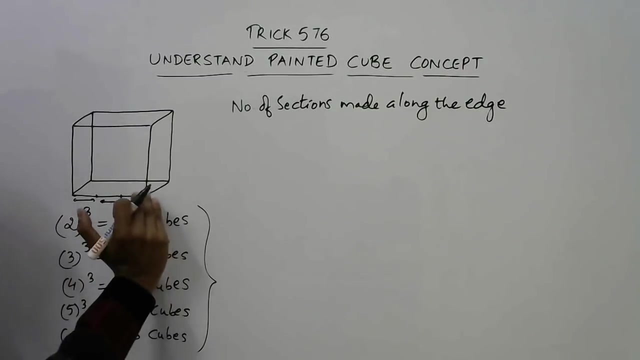 124,, 225,, 216 and other perfect cube numbers. Now, after this, the number of sections made along the edge. I am talking of the number of parts in which the length is divided here, or the number of cubes cut along the length, If you assume this. 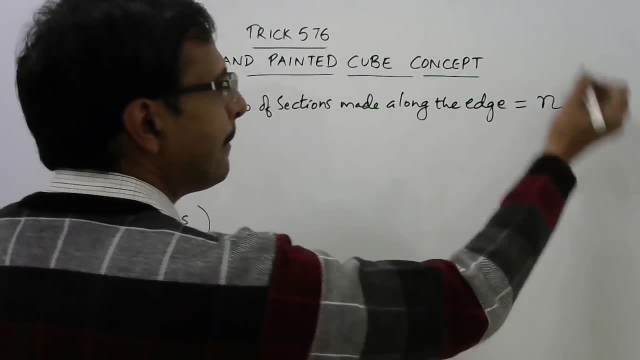 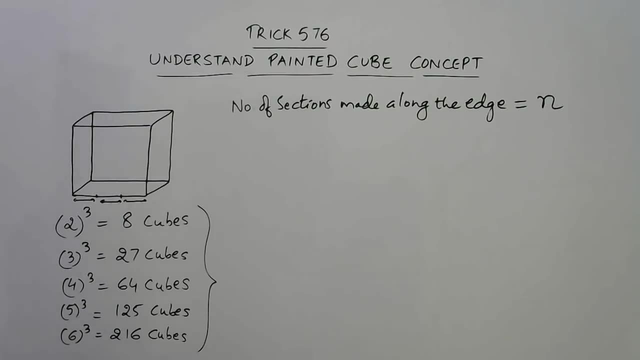 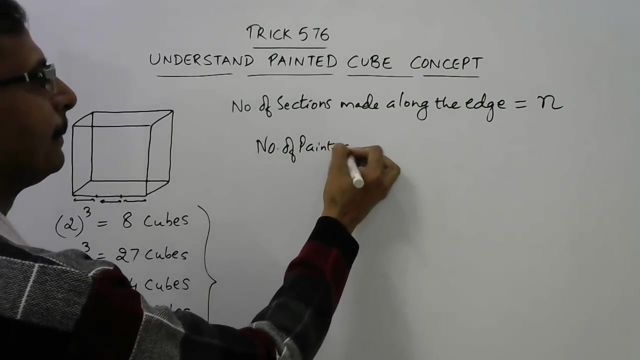 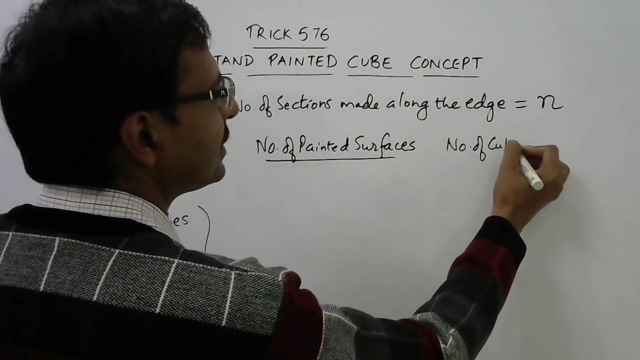 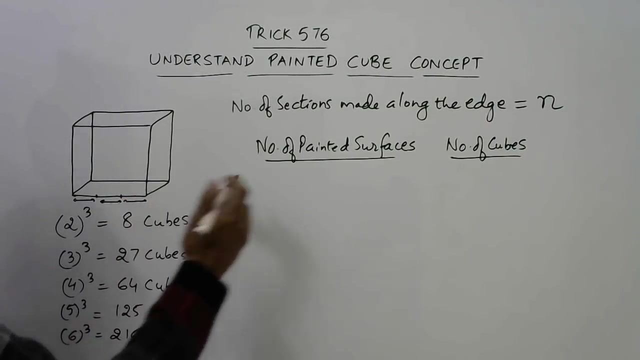 number of sections made along the edge be n. then, out of all these cubes, how many cubes will have three surfaces painted? Number of painted surfaces. this is first column and number of cubes the second column. Now I will tell you the short cut for this, See number of painted surfaces. 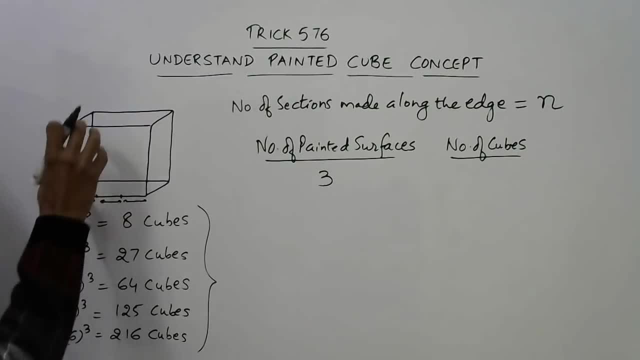 three. If you cut this in — along the length, breadth and height into smaller cubes, then some of the smaller cubes will have three painted surfaces. How to find how many cubes will have three painted surfaces? Now, this is important point. This is very important in Corner Scraper num日. 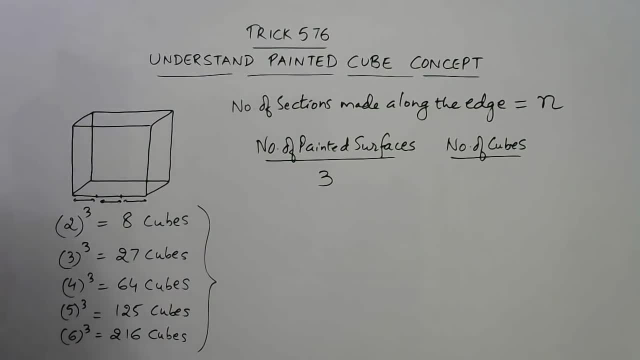 I don't know. Let me just go ahead and show it to you: surfaces. Let me tell you, let it be any number of smaller cubes, The number of cubes having 3 painted surfaces will always be 8.. Now, this is a fixed quantity, irrespective of the number. 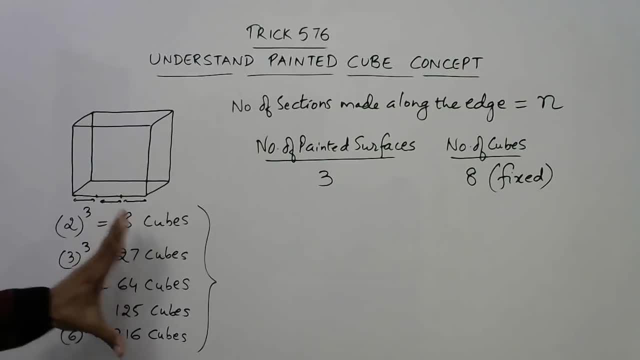 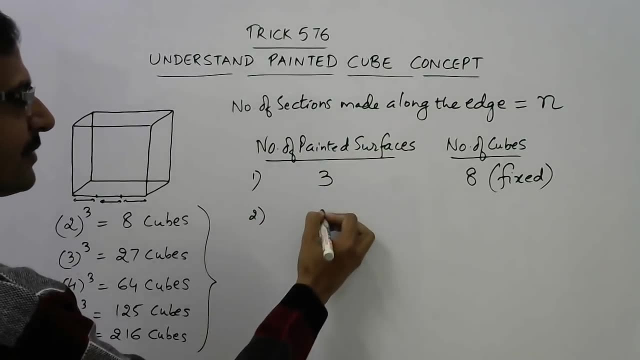 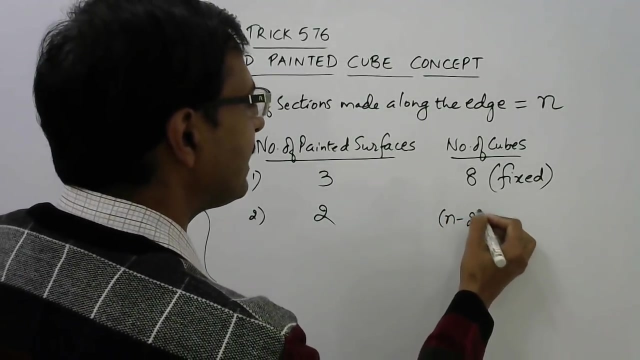 of cubes into which the larger cube is cut. What is the difference If the number of painted surfaces is 2, now you need to know: if there are 2 painted surfaces, the number of cubes having 2 painted surfaces will be n minus 2 multiplied by 12.. Now how to find this in. 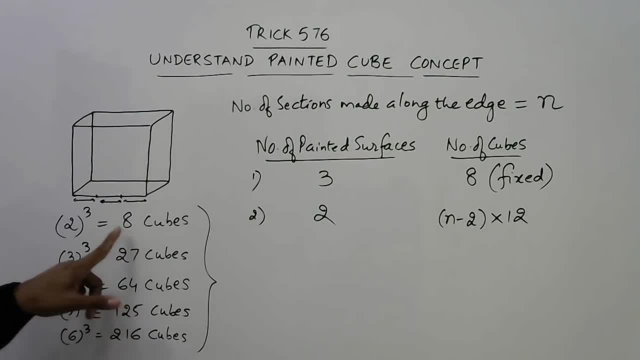 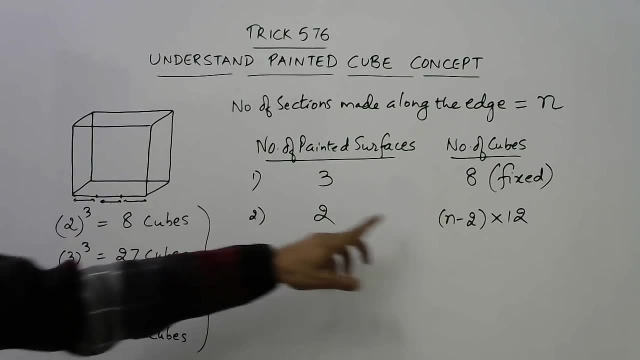 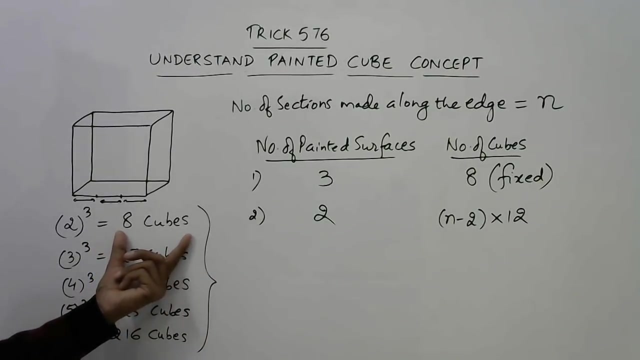 case of 8 cubes. Now, 8 cubes are made when the length is divided into 2 sections. So if you put n equal to 2 here, then this becomes 0. That means when there are 8 cubes made, then there will not be any cube having 2 painted surfaces. So you can just substitute n equal. 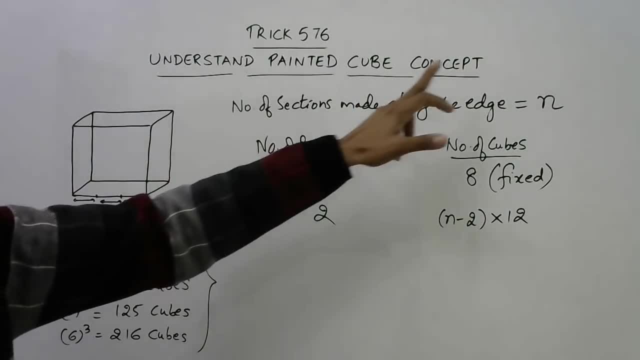 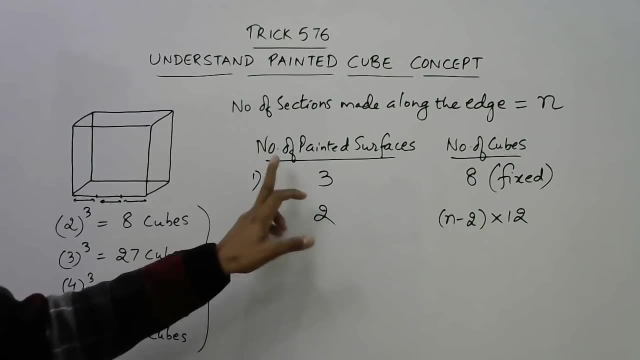 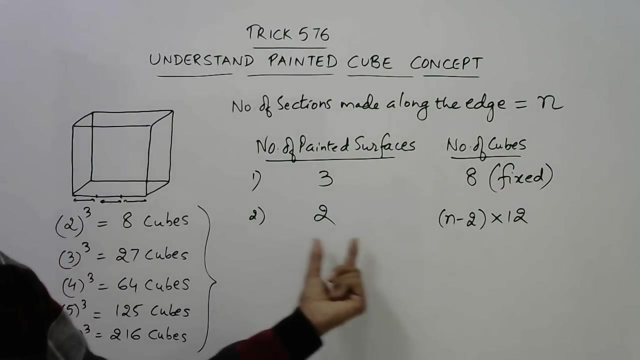 to 2, that is number of sections made along the length. So n is 2 means number of painted surfaces. Likewise, if the number of smaller cubes along the length is 3, just put 3 here, 3 minus 2 is 1, 1 into 12 is 12.. So there will be 12 small cubes having 2 painted surfaces. 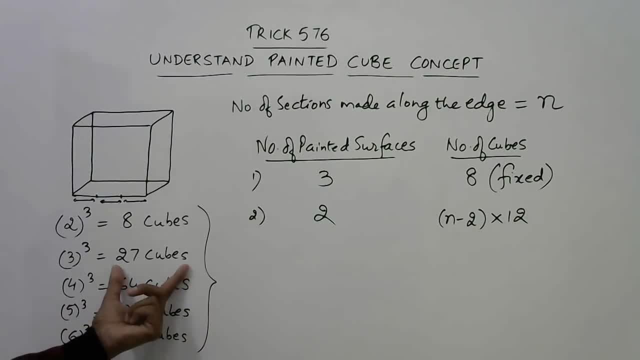 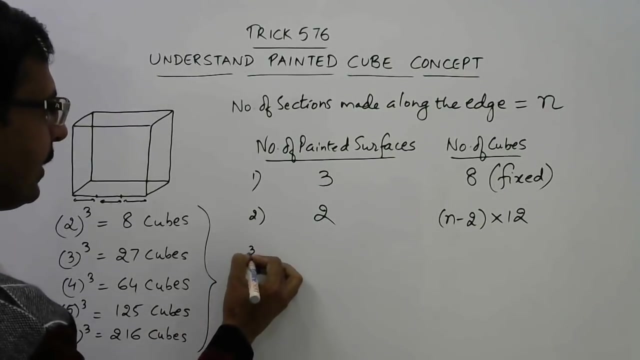 This is in case of 27 cubes. Out of 27,, 8 will have 3 painted surfaces and 12 will have 2 painted surfaces. So you can just substitute value of n from this base. Now the third one: How many cubes will have 1 painted surface? Now, 1 painted surface. 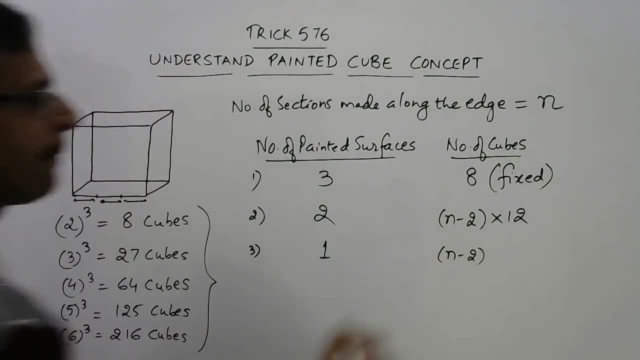 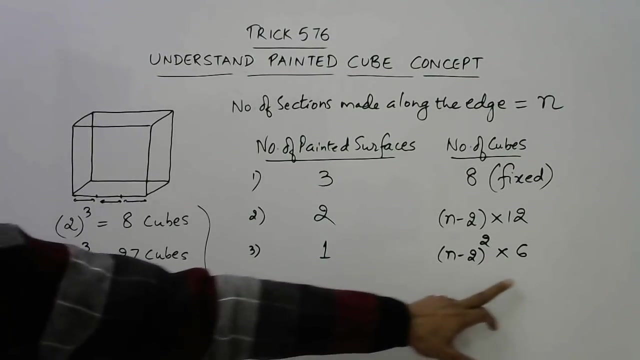 you can just write this n minus 2 again, but this time you need to find the square of this and multiply it by 6.. Now again, if there are 8 cubes, then n is 2.. Substitute n equal to 2, you get 0 again. 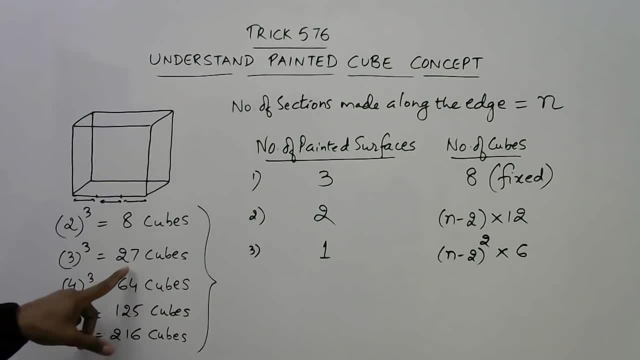 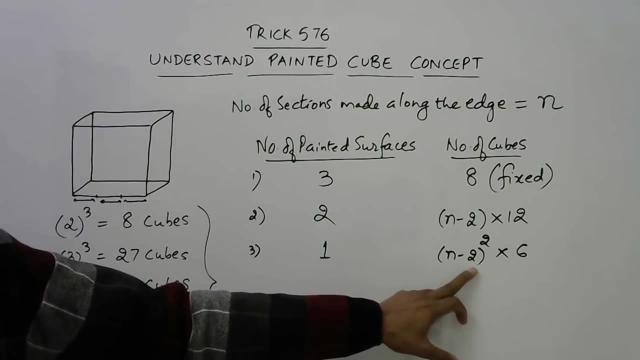 painted from three sides. But in case of 27 cubes, n equal to 3. put n equal to 3 here, 3 minus 2 is 1, 1 square is 1, 1 into 6, 6. So there will be 6 cube out of 27 which will have. 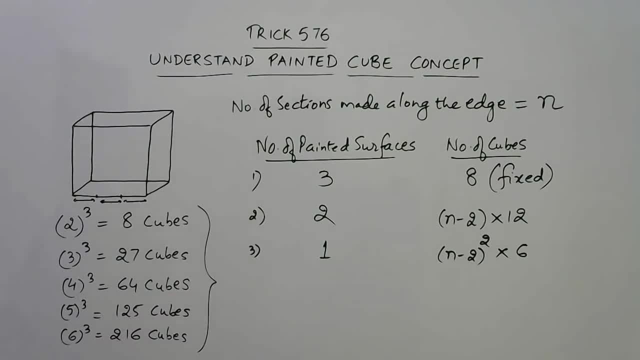 one painted surface. And finally, how many cubes will have no painted surface? Yes, Now again write the same factor n minus 2, and this time find a cube of this factor n minus 2.. So again, in case of 8 cubes, n is 2.. So there will not be any painted surface. 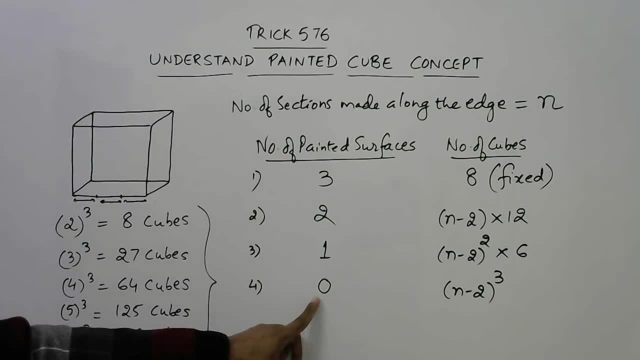 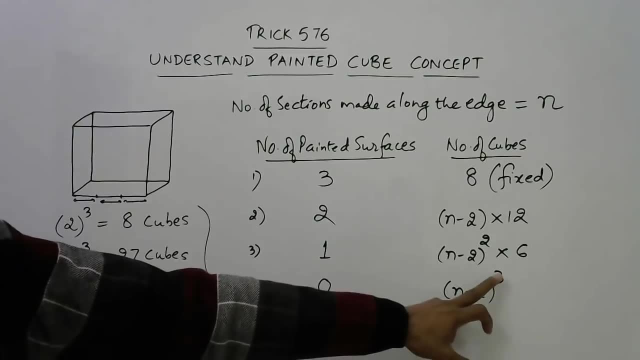 there will not be any cube which is not painted from any side. But in case of n equal to 3, that is 27 small cubes, 3 minus 2, 1, 1 cube is 1.. So there will be. 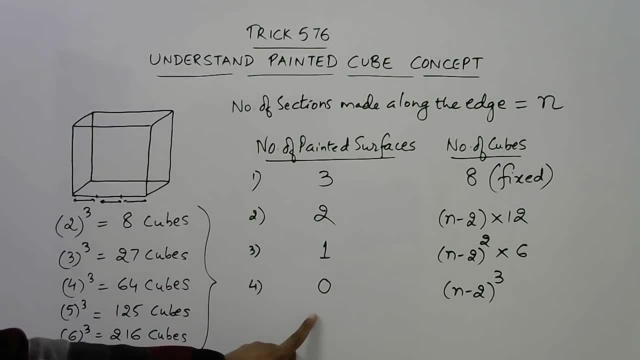 1 cube out of 27 small cubes. So there will be 1 cube out of 27 small cubes. So there will be 1 cube which will have 0 painted surfaces. So you can test this out. I will just find it for. 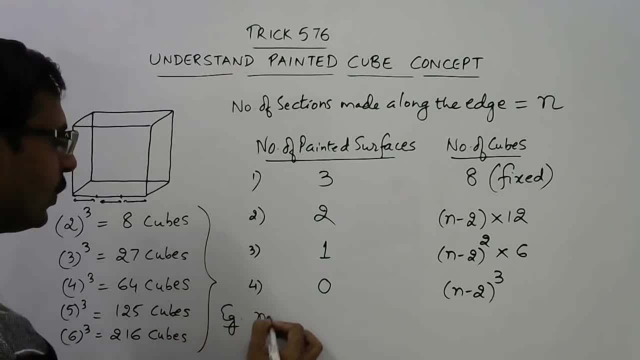 for an example I will take n equal to 4. that means 64 small cubes. So if a large cube is painted from all sides and then that large cube is cut into 64 small cubes, then we need to find how many of those 64 cubes will have 0 painted surfaces, 1 painted surface, 2 painted and 3. 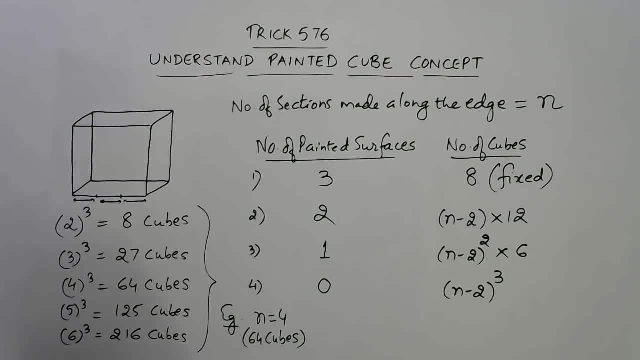 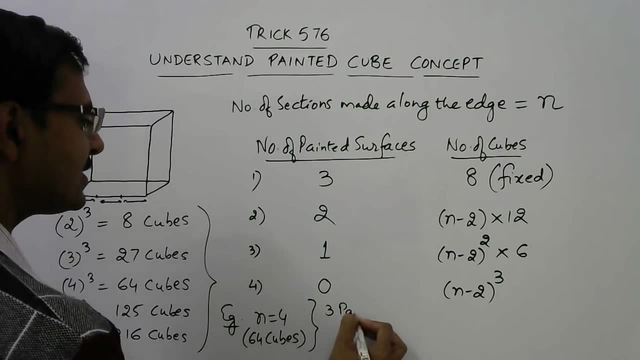 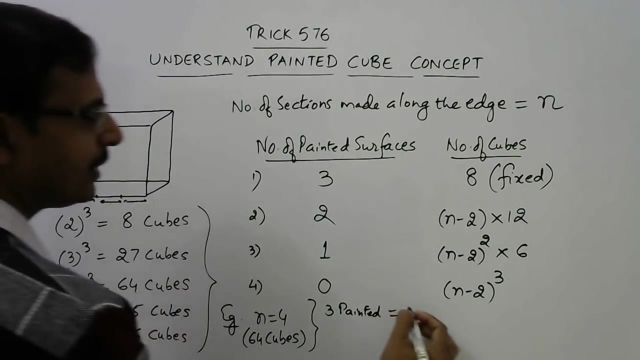 painted. Let us see In case of 64 cubes, n is 4.. So 3 painted surfaces, 3 painted are always fixed. So out of 64,, 8 will have 3 painted surfaces. Now let us talk of 2 painted surfaces. 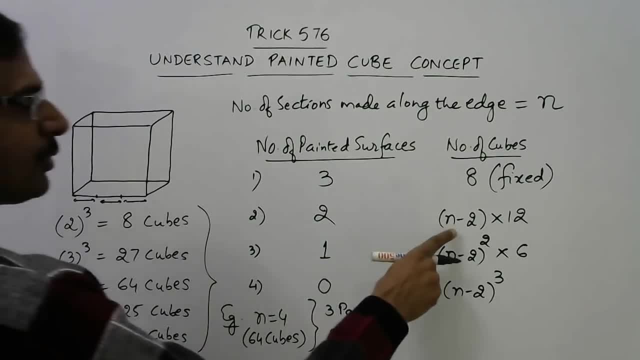 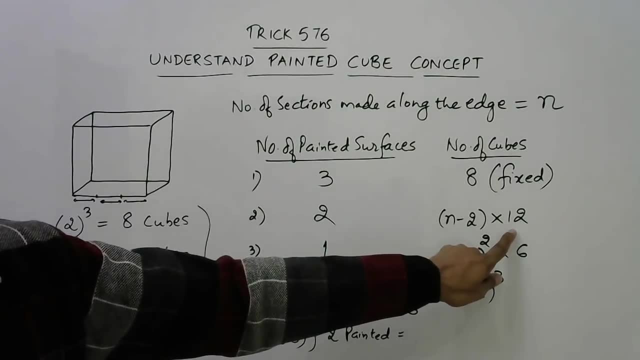 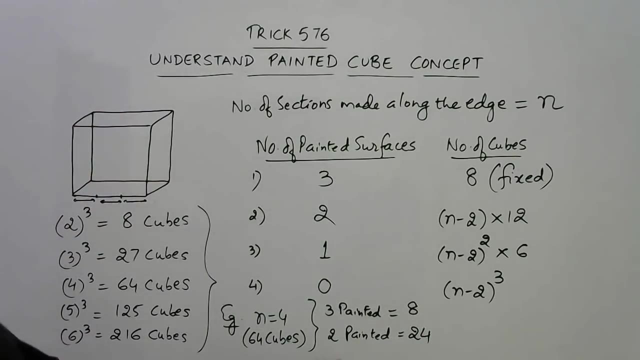 Here n is 4.. So just put n equal to 4 here you get 4 minus 2, 2 and 2 into 12, 24.. So we will have 24 cubes which have 2 painted surfaces out of 6.. Friends, you do not need to think about. 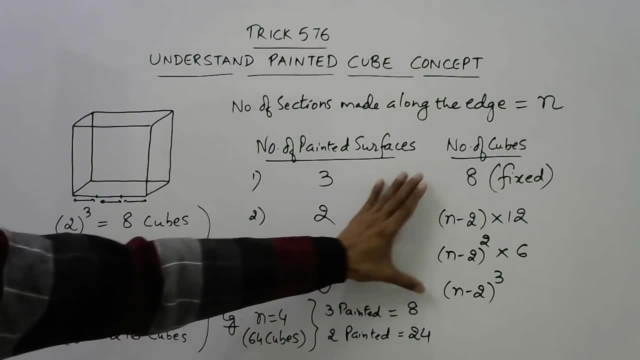 each of these. So let us talk of 2 painted surfaces. So let us talk of 2 painted surfaces. So let us talk of 22 color refrigerators. what is water proof? n is 14 cork, which is 3 c c, goodbye. 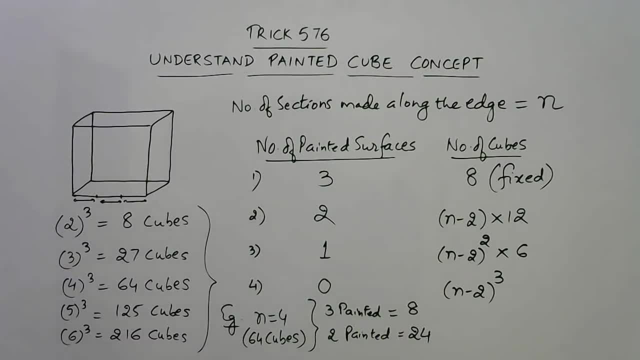 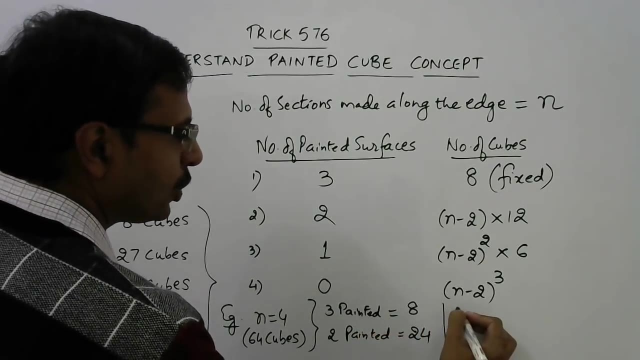 and slightly morgan F, but 1 freed surface, 1 free surface. so 1 freed surface, Each cube independently. You just need to know the concept, the shortcut idea, the formula, And here you are with the problem. if you start counting 24 cubes in exam in competitions, obviously a lot of time will be wasted. but those who know the formula, they will do it in hardly two second's time. 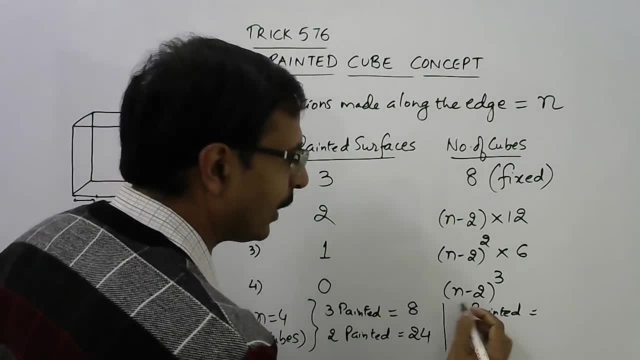 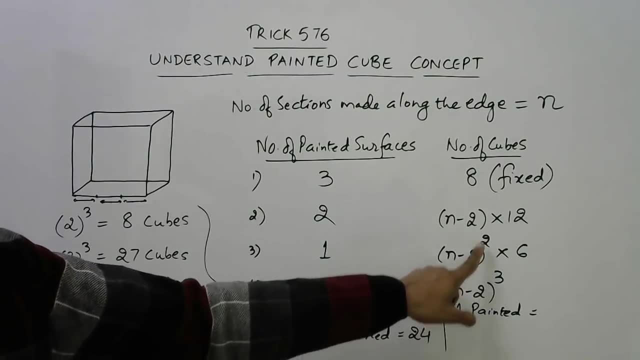 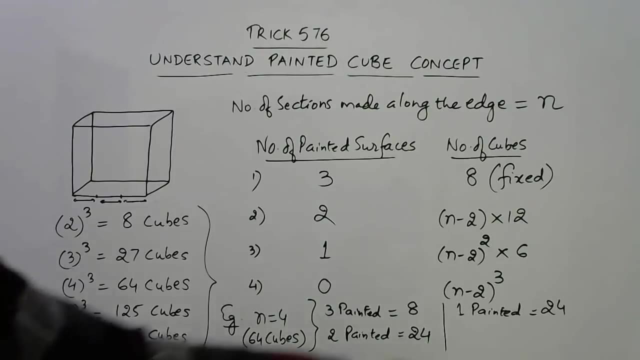 So we have done 2, let us have 1, 1 painted surface. ok, Now put n equal to 4 here. 4 minus 2, 2, 2 square is 4, 4, 6 are 24.. So again we have 24 small cubes which have. 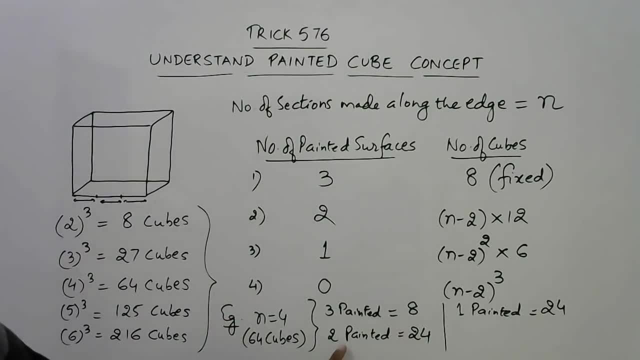 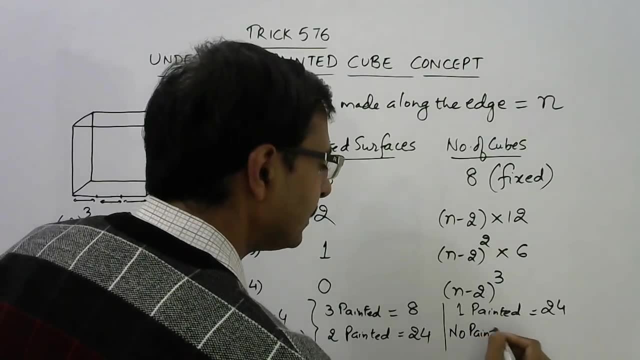 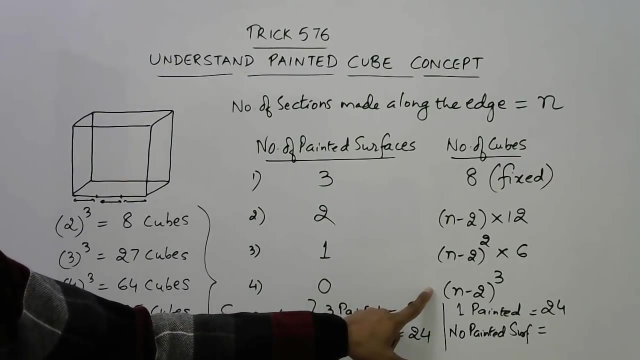 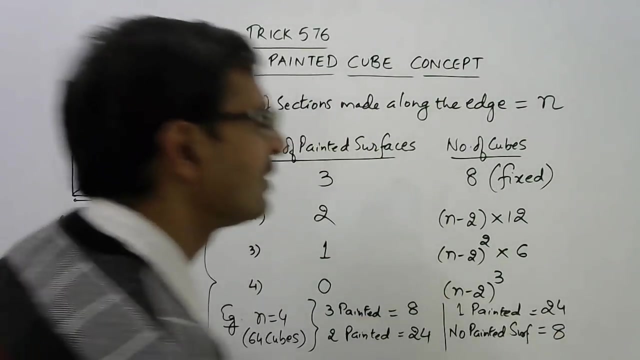 1 painted surfaces, 24 which have 2 painted, 8 which have 3 painted surfaces. And what about no painted surface? Let us see no painted surface. the formula is n minus 2 whole cube. put n equal to 4, 4 minus 2, 2, 2 cube is 8.. So we will have 8 cubes which have 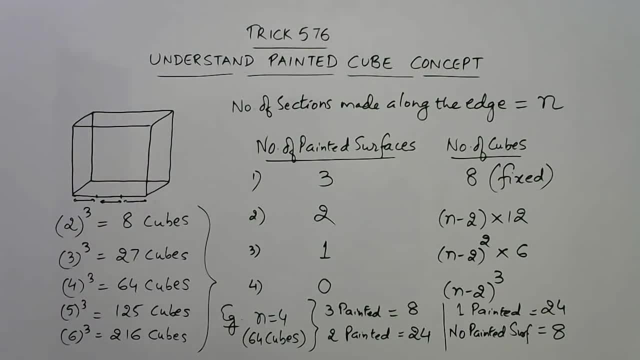 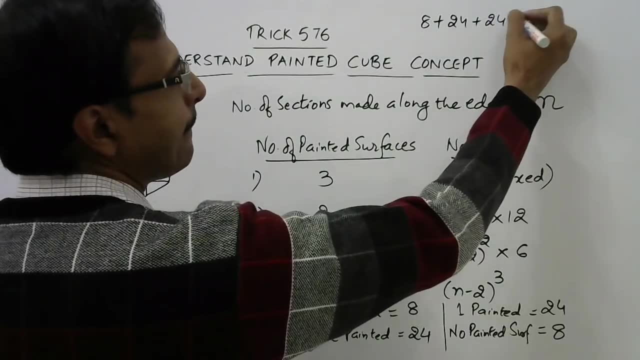 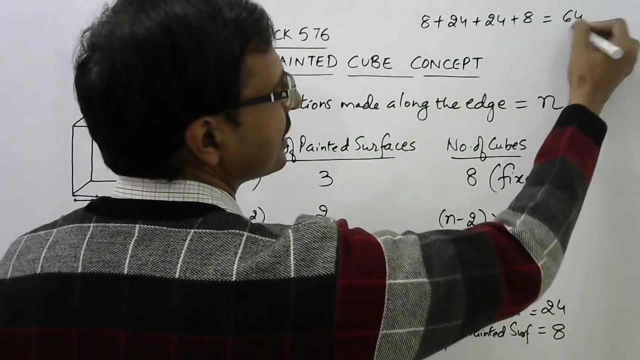 0 painted surfaces. Now let us verify this: 8 plus 24 plus 24 plus 8. This is 16 plus 24,, 40 plus 24,, 64 cubes. And here we are with the problem: out of these 64 cubes.